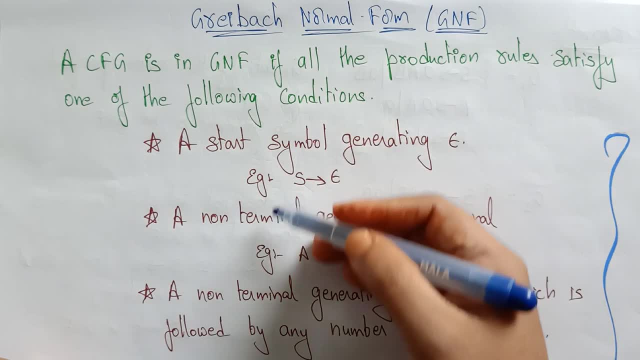 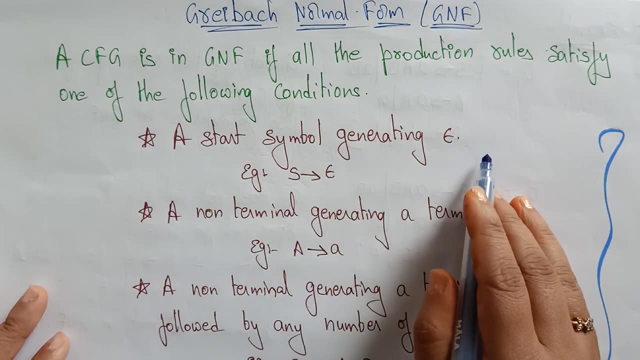 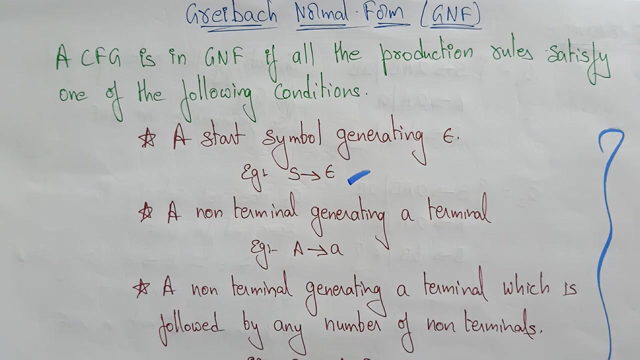 grammar. in that context-free grammar, it has to follow any one of these conditions. Let's see what are these conditions: A star symbol generating epsilon. So whatever the star symbol that is there that it can generate epsilon, Then you can say that the that a. 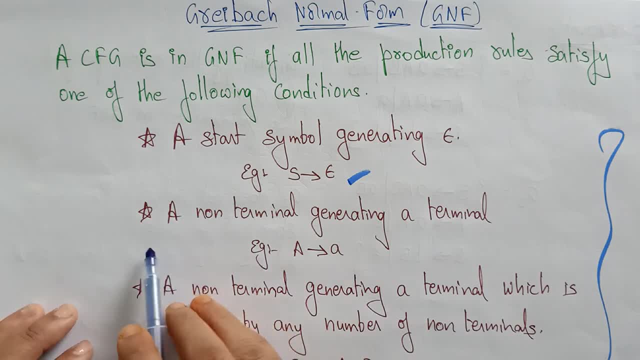 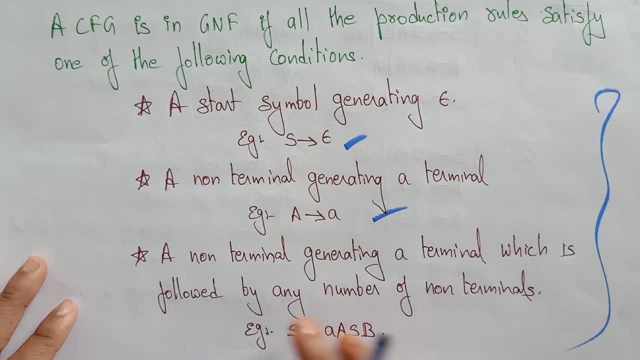 particular condition is a GRIBAC normal form. So let's see what are these conditions. Another production is in GNF GRIBAC normal form. A non-terminal generating a terminal. Okay, a non-terminal is generating a terminal. And the third one is a non-terminal generating. 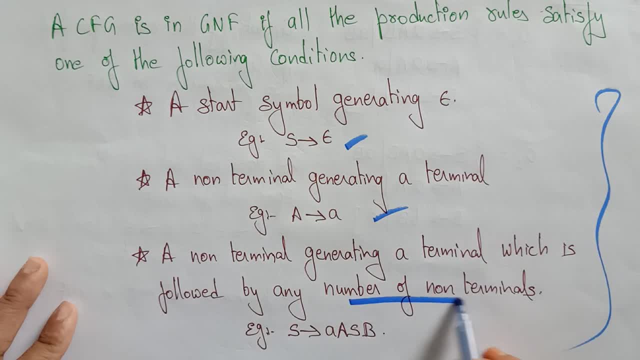 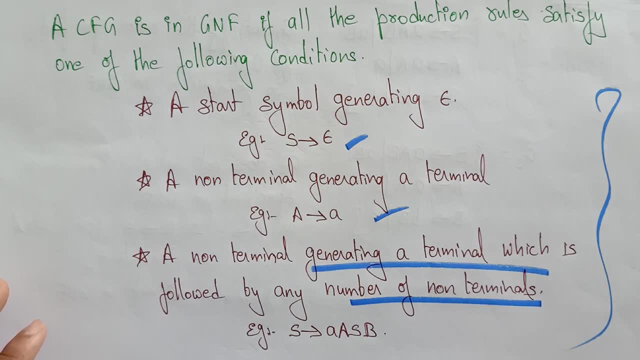 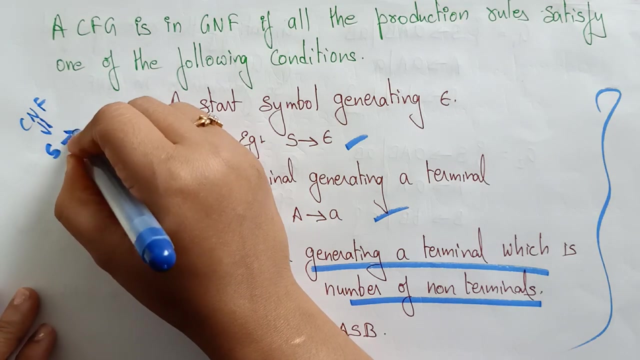 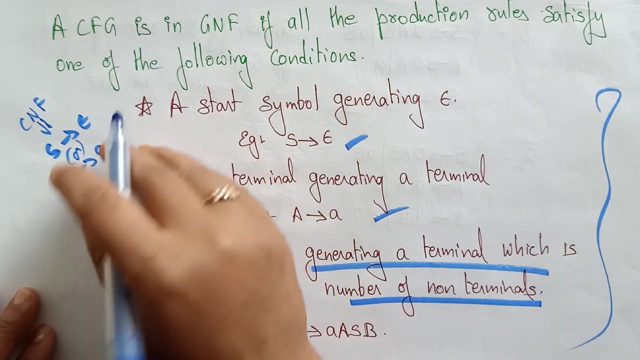 a terminal which is followed by any number of non-terminal. So this is the only difference between the Chomsky normal form and the GRIBAC normal form. Okay, in the Chomsky normal form, the star symbol is going to generate a. the star symbol is generating an epsilon, or a non-terminal is generating a terminal, or 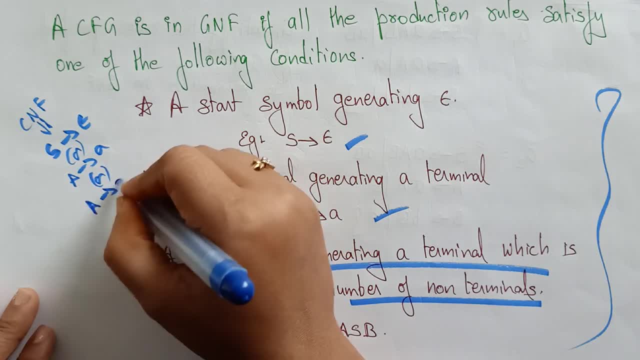 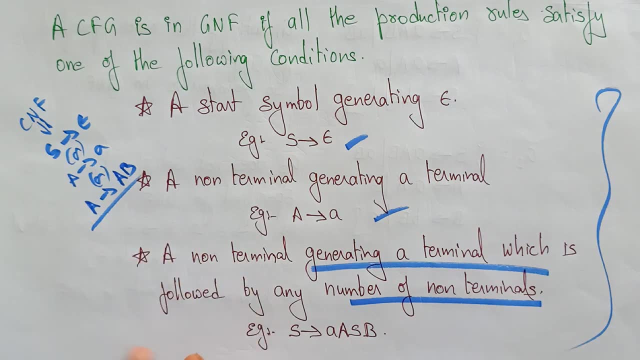 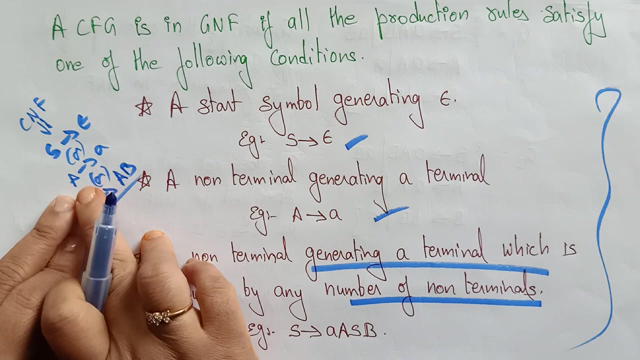 a non-terminal is generating more than it's only two non-terminals, not more than it's only two non-terminals should be there. So this is Chomsky normal form, Whereas GRIBAC, normal form, a star symbol is generating epsilon or a non-terminal is generating a terminal. So these two conditions. are satisfying. And the third one is a GRIBAC normal form. So this is the only difference between the Chomsky normal form and the GRIBAC normal form. So this is the only difference between the Chomsky normal form and the GRIBAC normal form. So these two conditions are satisfying. 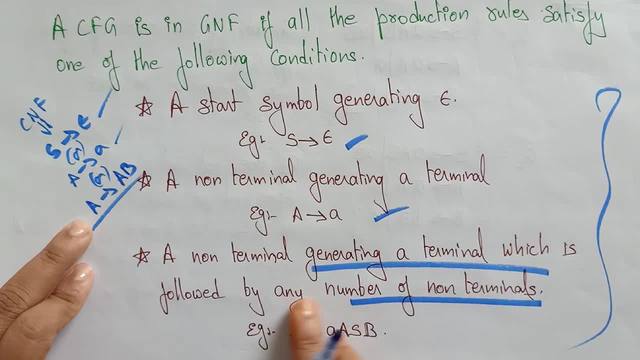 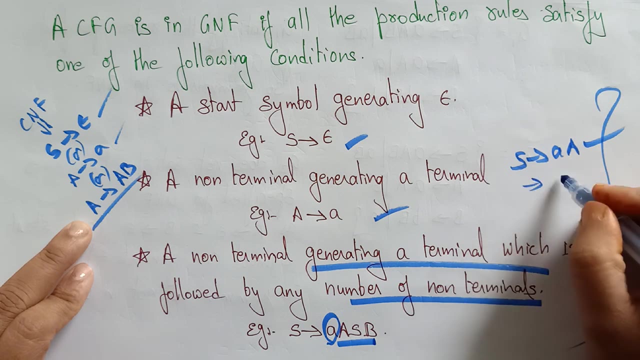 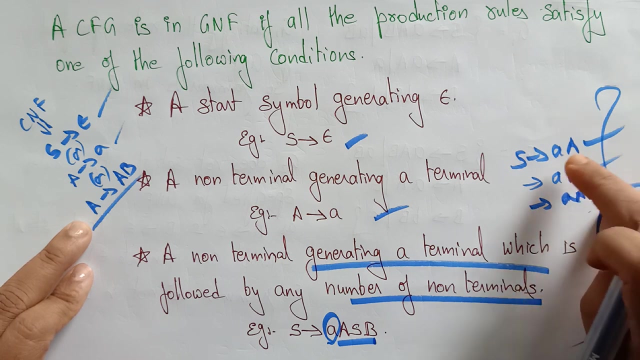 Here a non-terminal which is followed by it's generating a terminal. Okay, one terminal is generating and it is followed by more. any number of non-terminals means here it can this, this is in GNF. Okay, either this is in GNF or this is also in GNF means a non-terminal which is followed by: 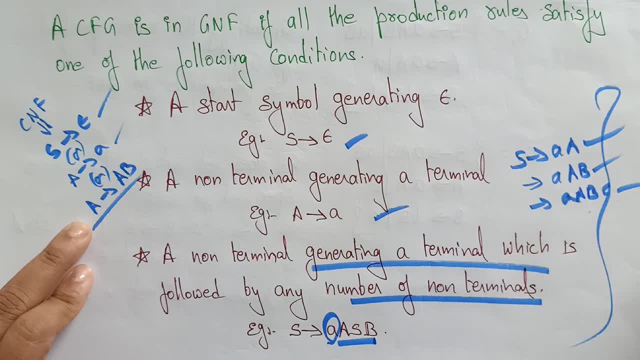 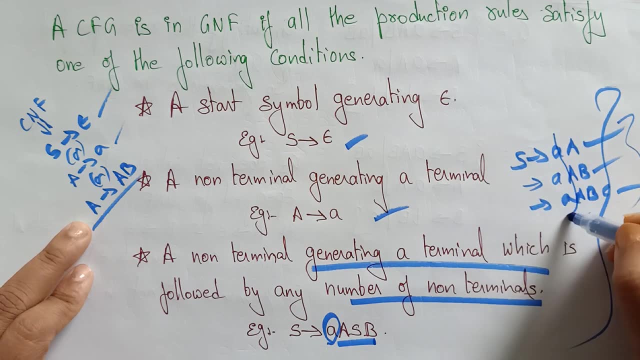 any number of non-terminals followed with any number of non-terminal. then we can say that is in GNF, GRIBAC normal form. The only thing is the starting symbol should be a terminal, followed by any number of non-terminals. 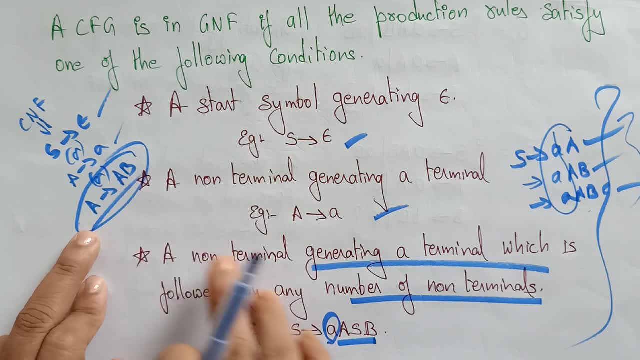 Okay, so this is a main difference between here. this is: this condition is violating here in the GNF, because the start symbol on the right hand side should be a terminal, followed with any number of non-terminals, But here the start symbol, the start symbol of this right hand side, should be. 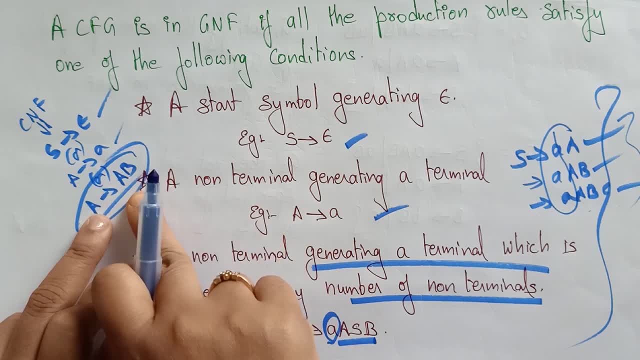 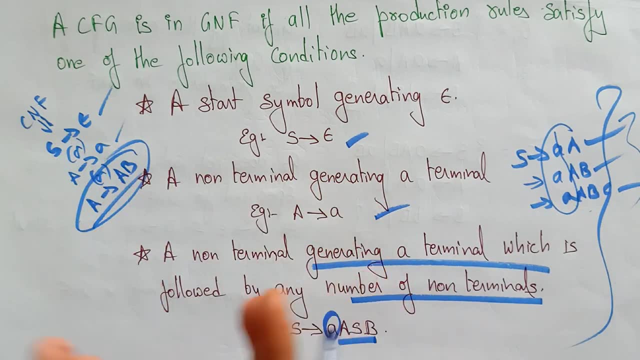 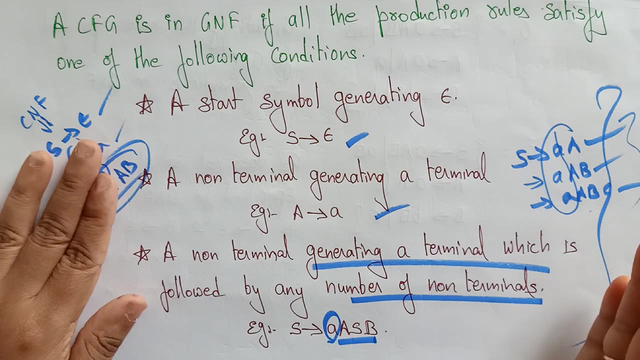 only either single terminal or it should be a two non-terminals. that is CNF. Okay, so here just concentrate on GRIBAC. If you want any confusion, just compare the CNF and GNF. So the context-free grammar is in GNF, When you say that the given context-free grammar is in GRIBAC, normal form. 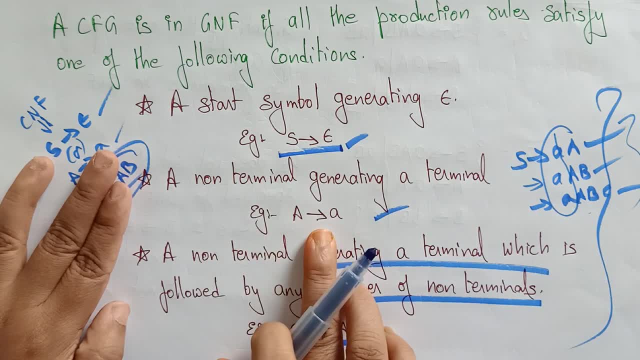 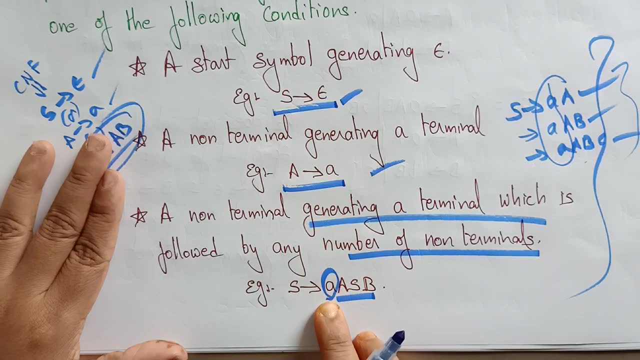 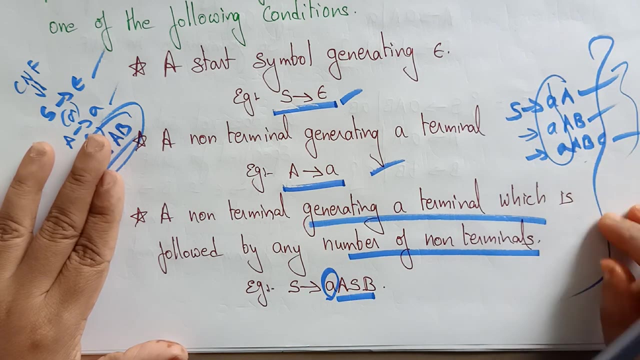 whenever the start symbol is generating an epsilon. one rule and the non-terminals is generating a terminal. and the third condition is a non-terminal is generating a terminal. Okay, a single terminal which is followed by any number of non-terminals- any number, 1,, 2,, 3,, 4,, 5, 6, any number- but it should be followed with means. the starting should: 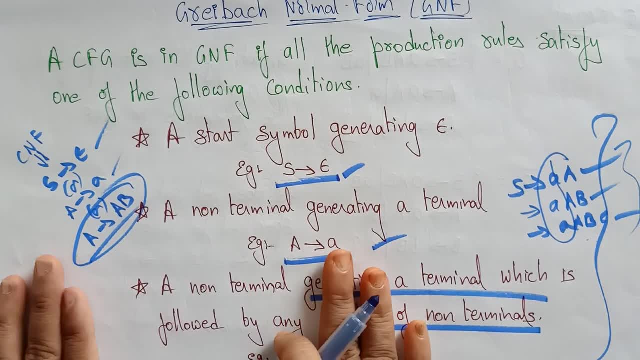 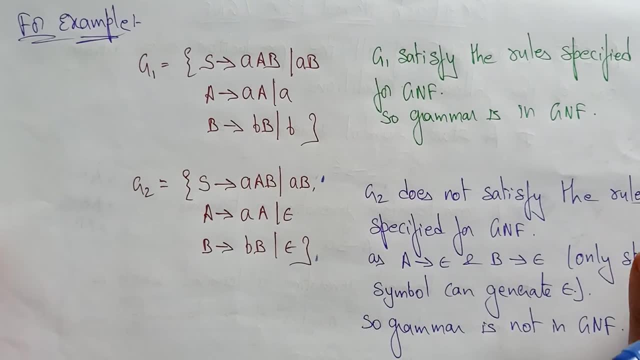 be a terminal should be there. So these are the conditions for the GRIBAC normal form. Let's see whether this grammar is in which grammar you can say that is in GNF and it is not in GNF. Let's see whether this grammar is in which grammar you can say that is in GNF and it is not in GNF. 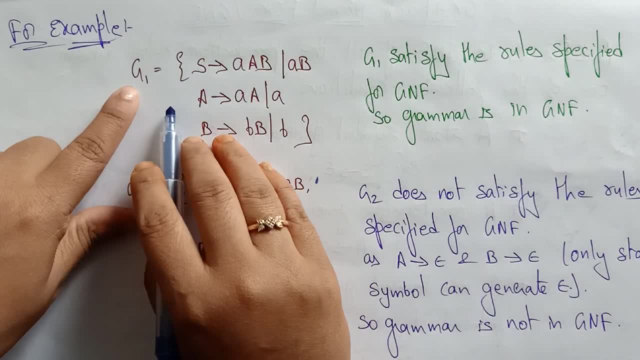 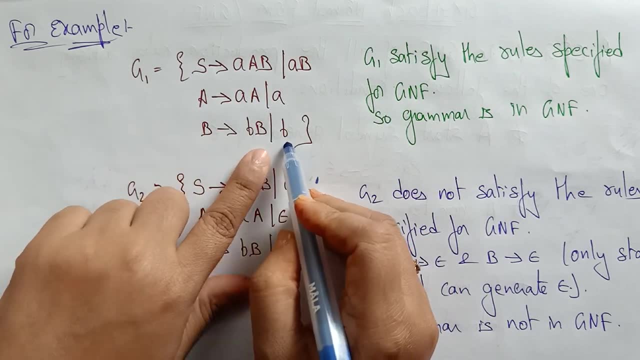 Let me consider two grammars: G1 and G2.. So in the G1, S determines AAB or AB, A determines AA or A and B determines BB. only Now I need to check whether this grammar is in GRIBAC normal form. 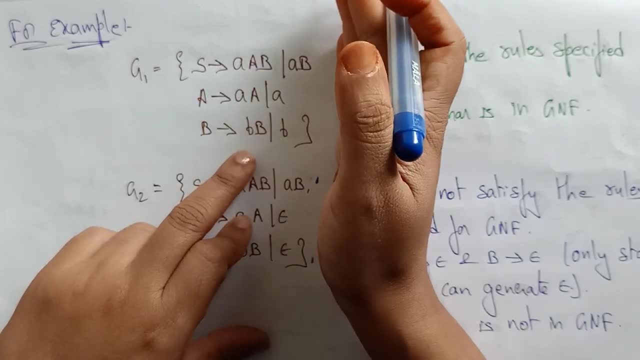 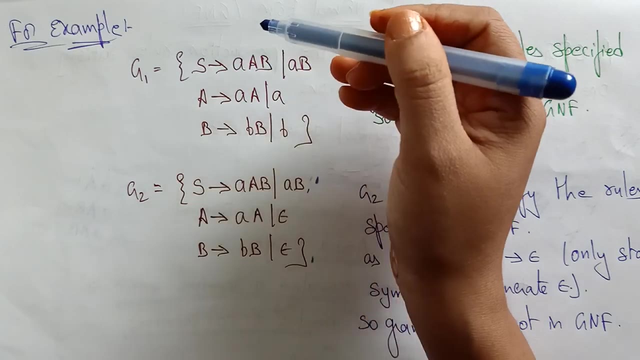 or not. First, I can clearly say this is not in CNF. How I can say it is not in CNF- because it is followed with the starting letter- is in: A. That is sorry, it is a terminal will be there. 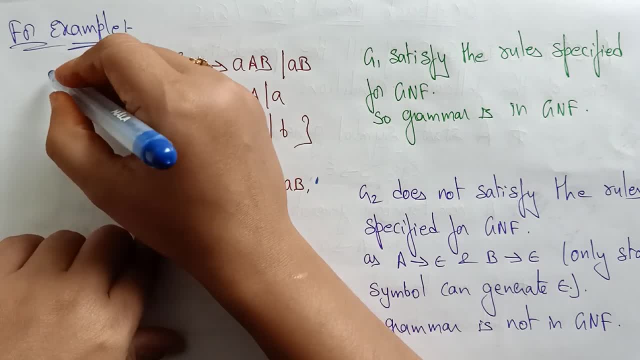 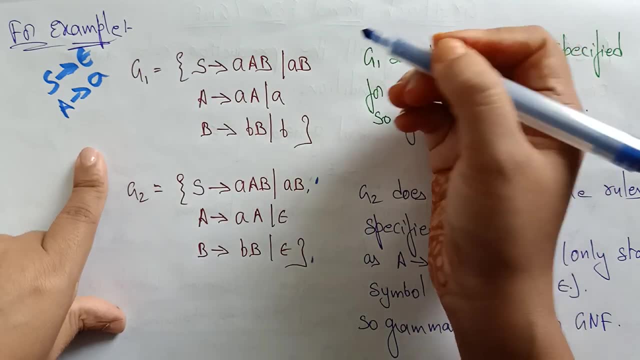 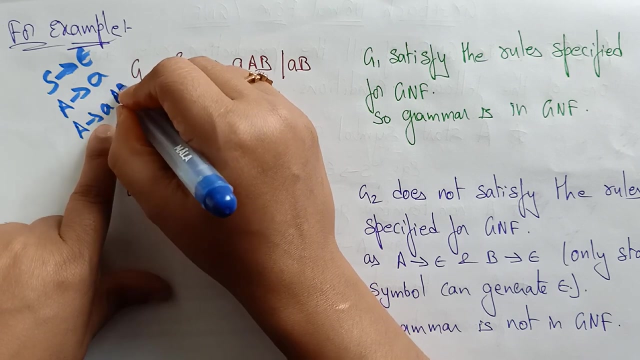 But now let me check the GNF. GNF rule means the start symbol should be epsilon, or a non-terminal is generating a terminal, or any non-terminal can be followed with A. The terminal is following with any number of non-terminals, A terminal is followed with any number of non-terminals. So 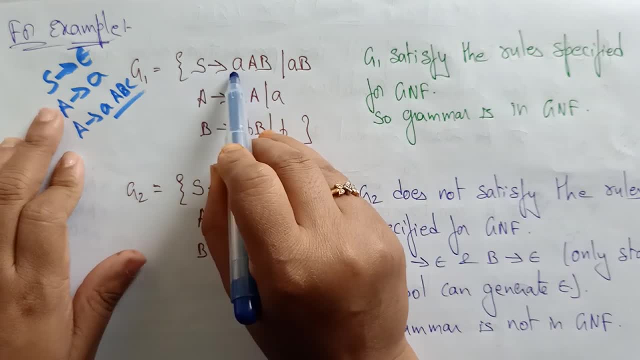 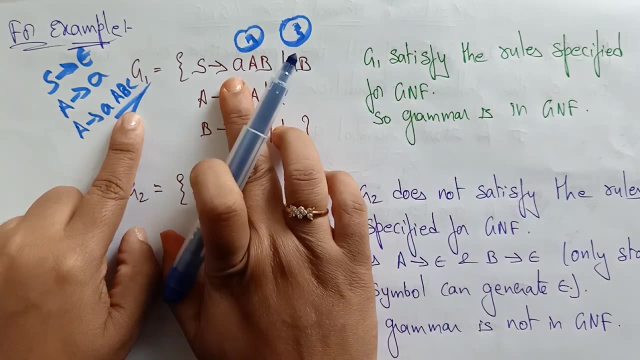 these are the rules for the GNF. Let's check whether it is following or not. S determines AAB. Okay, It is following And this is AB. This is also following rule 3 because the starting is a terminal, If terminal. 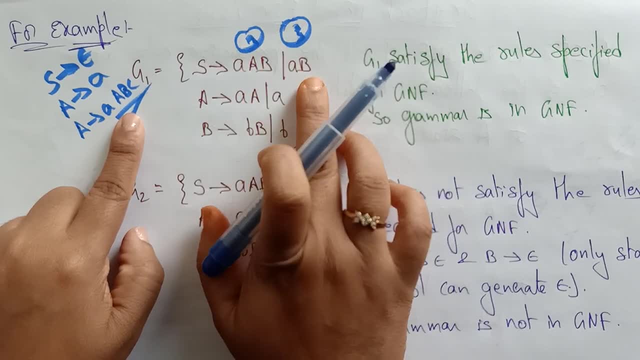 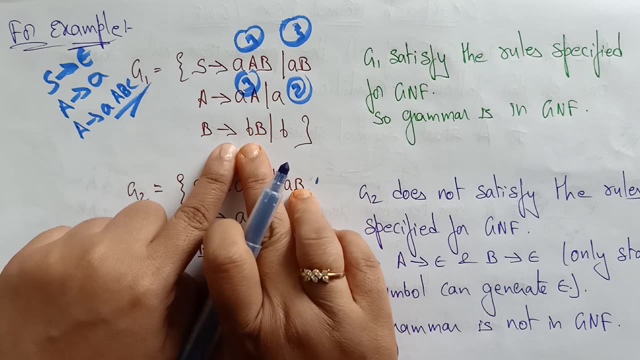 is there, followed with any number of non-terminals, then it is in GNF. Okay, So this is also following rule 3 and this is a rule 2.. A determines A and A determines BB. So this is also in rule 3 and